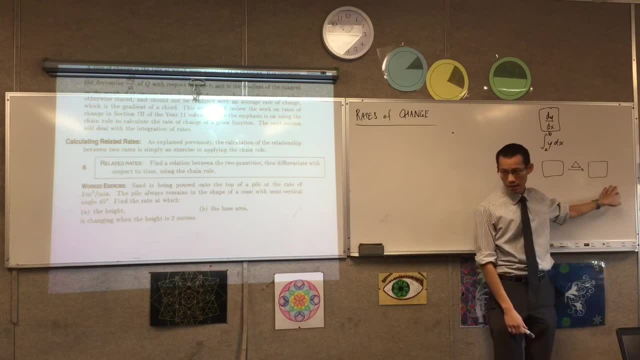 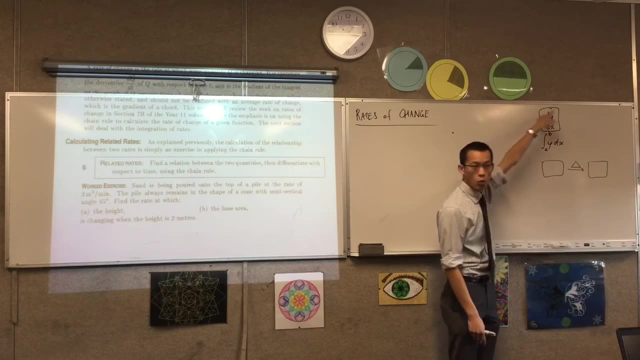 happens. usually the change is like heat or whatever it is, and then you get something out the other end. okay, So delta, the Greek letter delta corresponding to our little d, that's what that refers to. okay, Change in y. I want to compare that to the change in x. okay, Now, when we look, 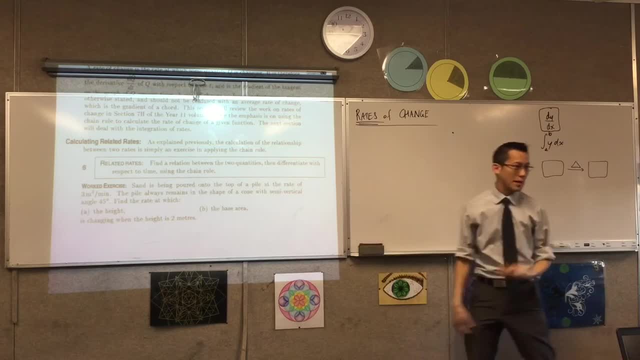 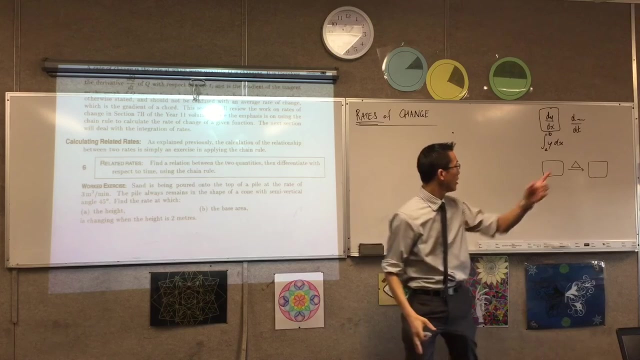 at the relative change. when you hear the word rate, basically, what you're meaning is something is changing over time, right? So instead of dy over dx, it's going to be d, something over dt, right? So I want to investigate how some particular quantity is changing. with respect, 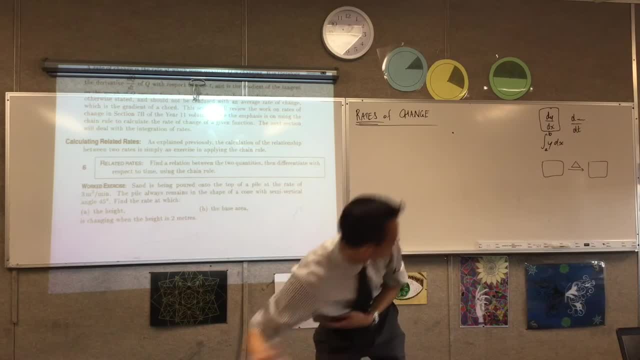 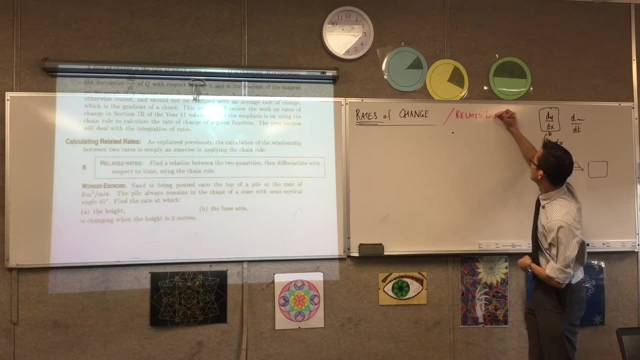 to time. okay, Now, what we add as extension one, students, is what are called related rates. The idea be- and here's an example- you've got different kinds of things within the situation that are all changing with respect to time, and these things are connected to each other, right? 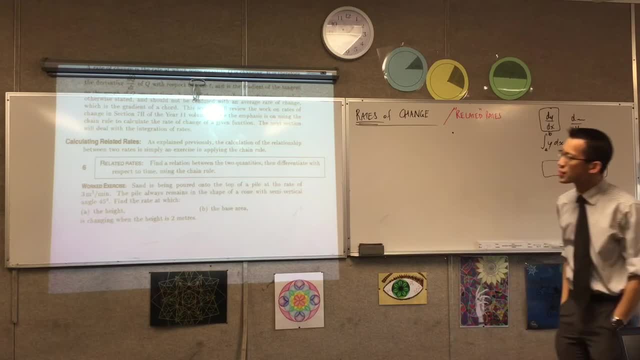 So let's actually have a look at this question, and then we'll start to unpack. The sand is being poured onto the top of a pile at the rate of, and then they give you a number. okay, So stop for a. 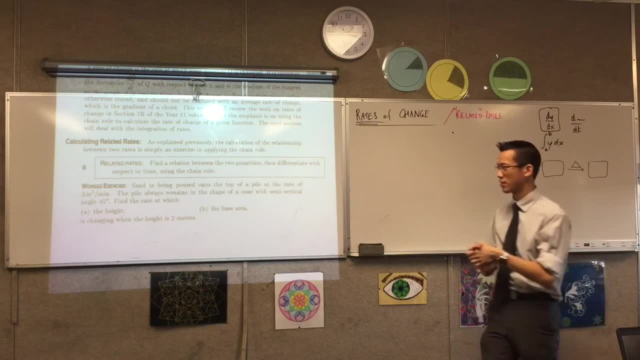 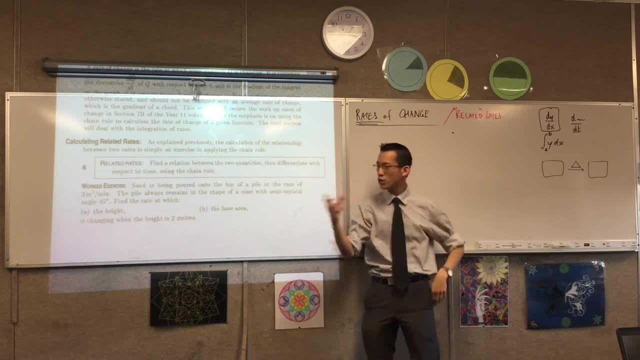 moment and just try to get a picture in your head. I hope you haven't looked at the next picture and sort of swore it for yourself. There is a point. there is a point. there is a pile of sand and it's growing and growing, and growing. Now, if you're just like 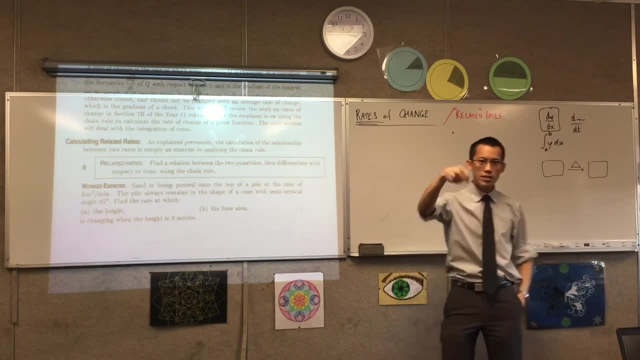 if you're not mucking around with it. you don't have like a bucket or something like that. what is the shape of this pile of sand as you're pouring right? Yeah, and it's going to be conical. 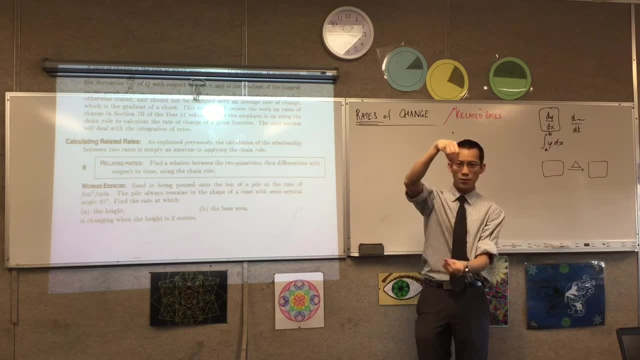 isn't it? Because it starts on this little spot and it grows up and up and up, but obviously because it's unstable, it can't just grow like a tower, okay. So it sort of just pans out like 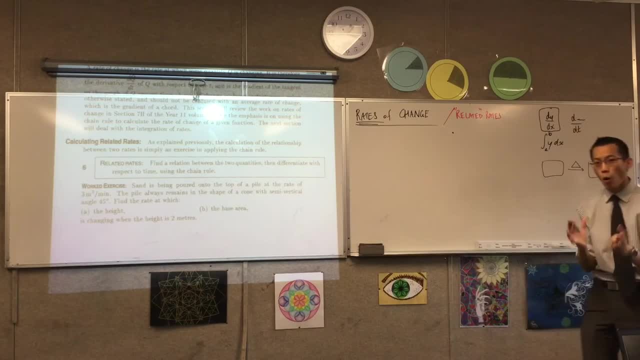 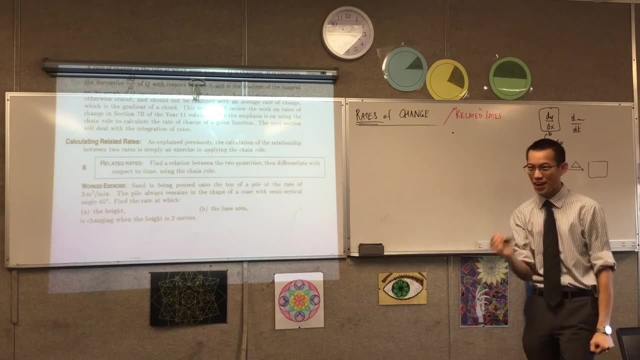 this. okay, So draw with me. let's draw a diagram and for all, rates of change questions, but particularly related rates questions, your diagram. you will live or die on the basis of your diagram. okay, So don't make this too small. 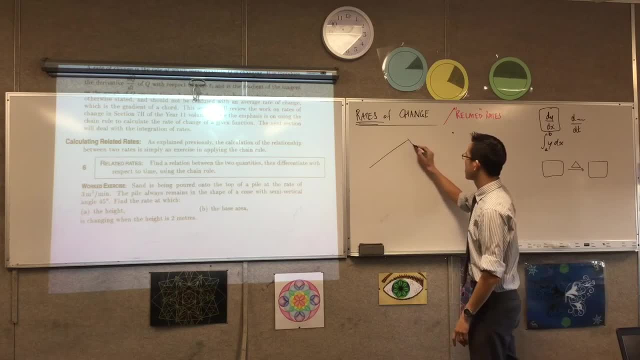 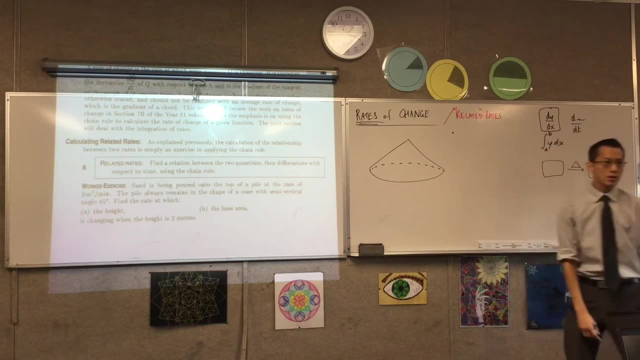 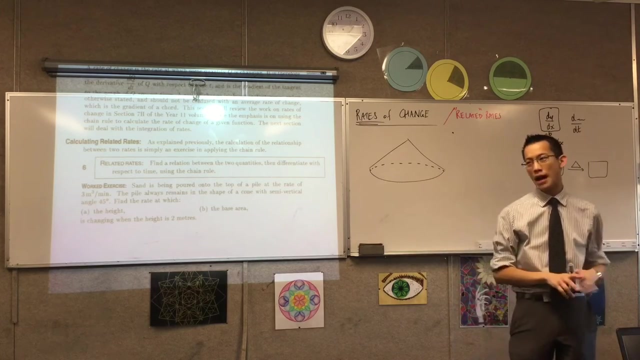 we're going to have to do some labelling on it, and so on. You suggested to me that there's going to be this conical shape, So here's my pile of sand. yep, And importantly, what I'm drawing here represents the pile of sand at an instant in time. So this pile of sand. 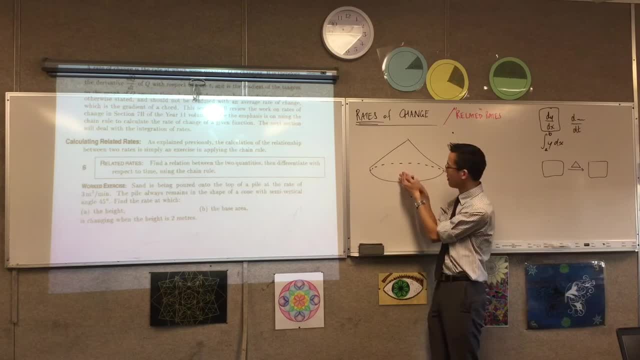 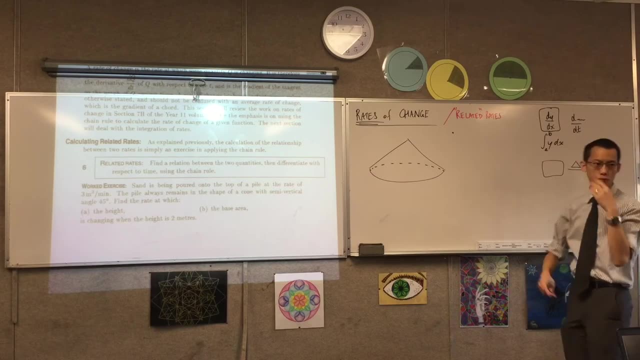 at some point in time it didn't exist. It was a tiny little dot and then further in time, it's going to get bigger, right? So this represents like I snapped a photo. okay, So I'm trying to represent change, but I have to do it in. 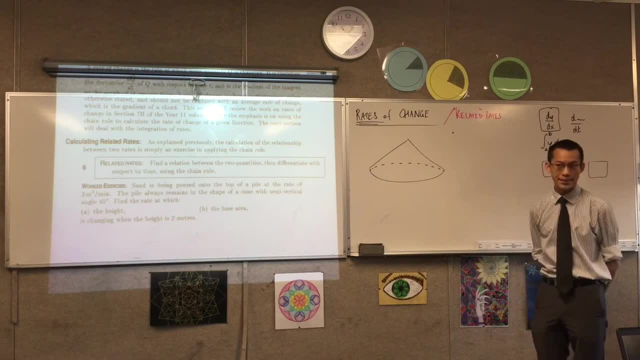 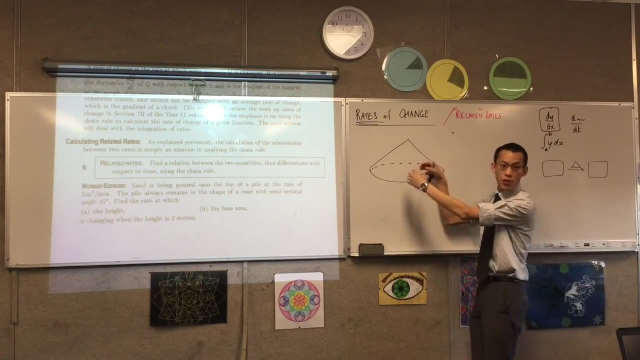 a static medium. So this is my pile of sand. at a particular moment It's being poured onto the top of a pile, so here comes the sand up here, and so this cone is getting larger and larger at the rate of three metres cubed per minute. Okay, let's just write that down for a second Three metres. 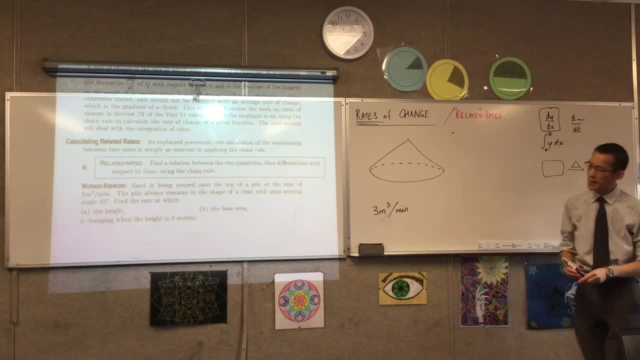 cubed per minute. Now you remember I said to you, in rates of change, land instead of d1 and dx. it'll be something on dt. You're going to get dt over and over and over again. And the way you can know is when you look at this, if I write this in the same form that I've got. 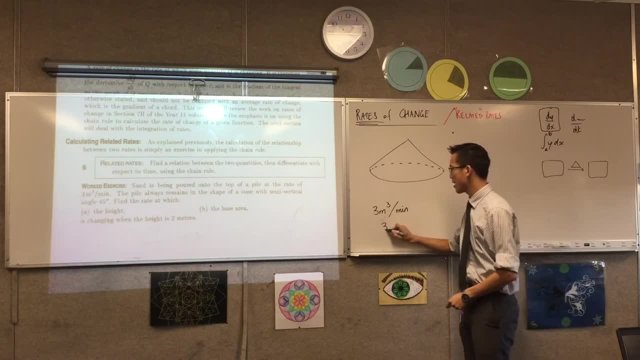 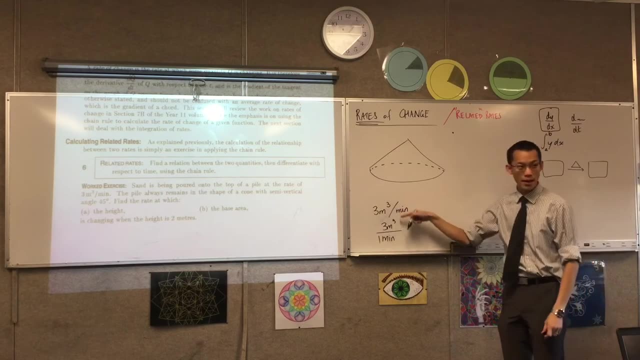 here, which it almost is right, I would write this as three metres cubed over one minute. really, When I say three metres per minute, I mean three metres, sorry, three metres cubed. three metres cubed per instant. 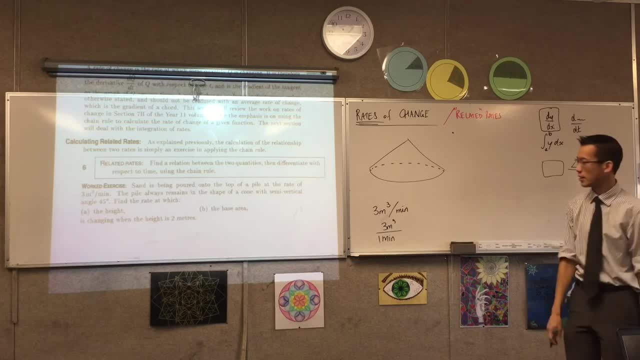 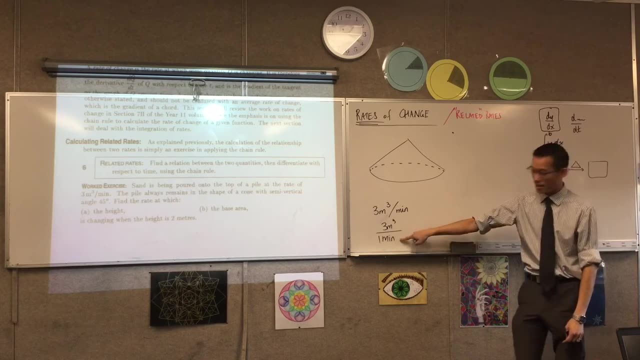 Okay, so that's the individual minute, right. So there's really a comparison of two units here, which is what makes it a rate And you can see here it tells you what it is right. This is our dt, because minutes are a unit of time. They could just as easily be hours. 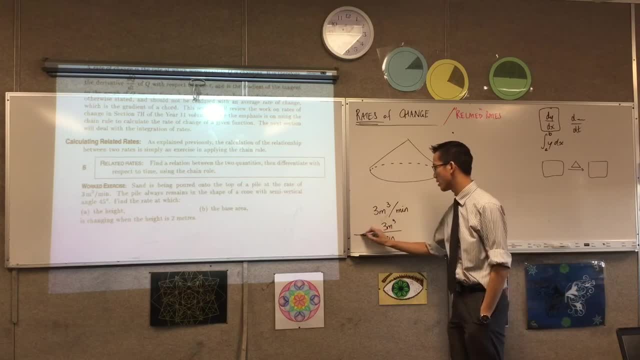 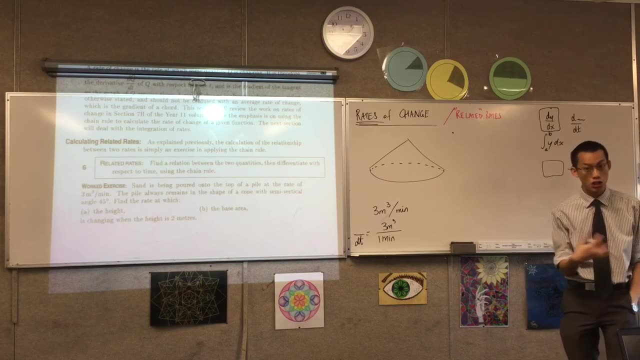 or days or seconds if you wanted to, So you can see. this is the dt on the bottom, Metres cubed. what's that a measure of? It's a unit of volume, isn't it? So up at the. 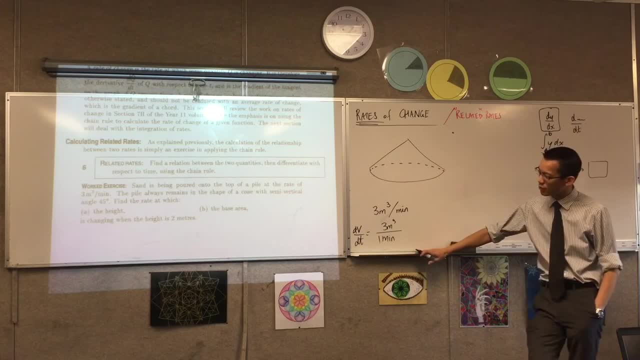 by convention, we usually use a capital V. We tend to reserve the lowercase v for velocity, which we'll talk about later. So this is my rate of change of the volume of the pile of sand And it's important because this is related rates and we're going to have 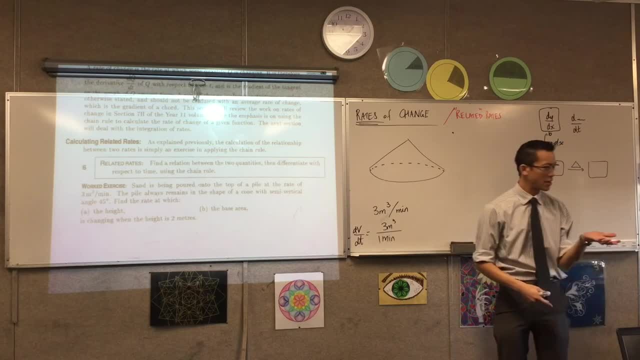 lots of different derivatives flying around. You remember I said to you right at the beginning, when people introduced this notation, and they also introduced this notation right Now that we're in related rates, land right, this dash notation becomes completely insufficient. 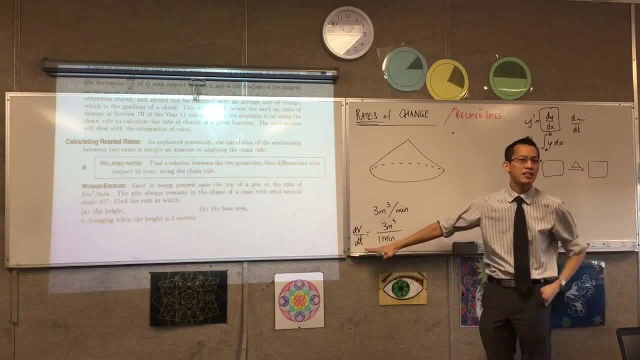 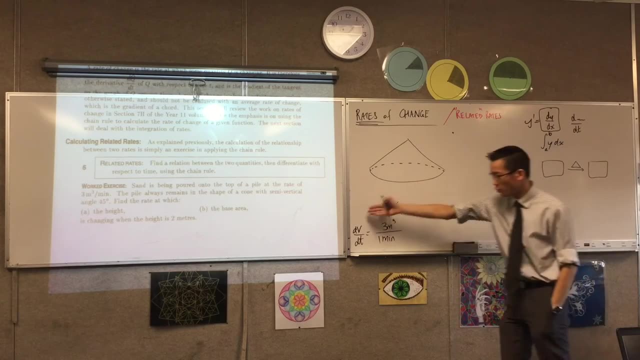 because it's kind of like what's being differentiated with respect to what? Just state it, Just state it. You're not really like people say, oh, it's faster, Not really Okay. So I've got a change of the volume. with respect to time, The pile always remains in the shape. 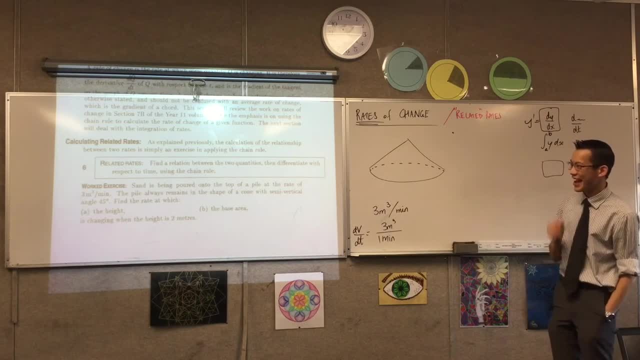 of a cone. I'm going to spoil this With semi-vertical angle: 45 degrees. Now, that's a bit of specific language there. So the semi-vertical angle, semi-vertical angle, it's half of some particular angle. Where is this angle? Where do you think it is? It's half of some particular angle. 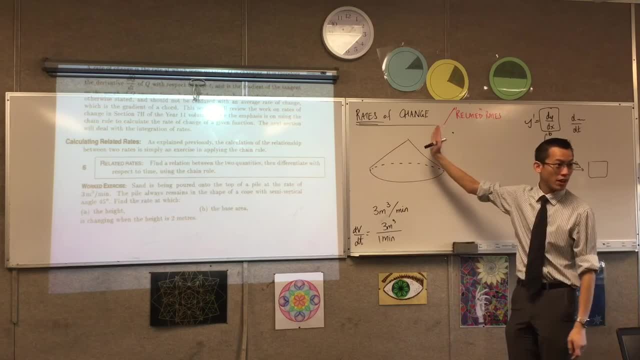 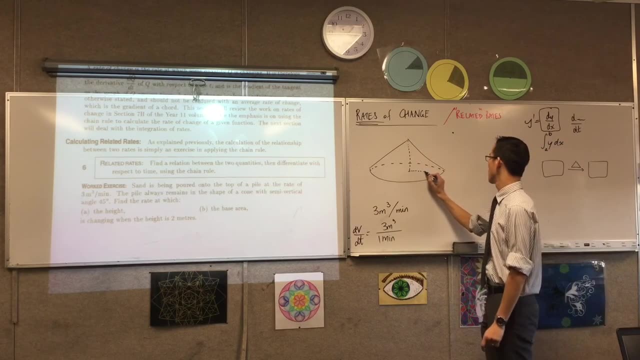 Okay, So that's half of some particular angle. Where is this angle? Where do you think it's going to be? Yeah, it's going to be up there at the top. yeah, So I'm going to actually put in a vertical line here, so it's perpendicular to the base, Like so, And the 45 degrees that. 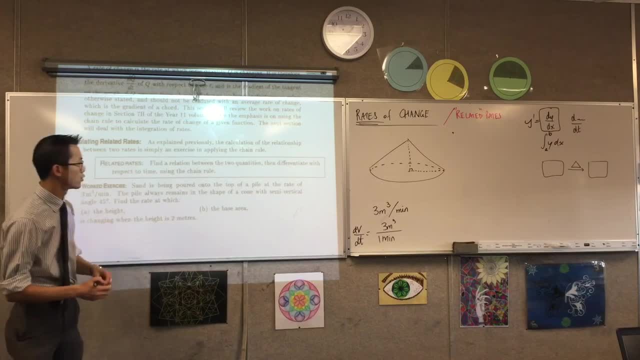 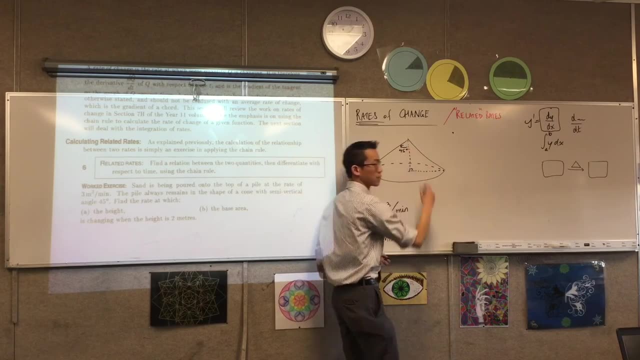 they're thinking of you, can I mean, in this case, you actually could draw it on either side, because 45 degrees is going to be equal, But what they really need is the inside angle here. How do you know that? Okay, How do you say that? Well, you're really describing the. 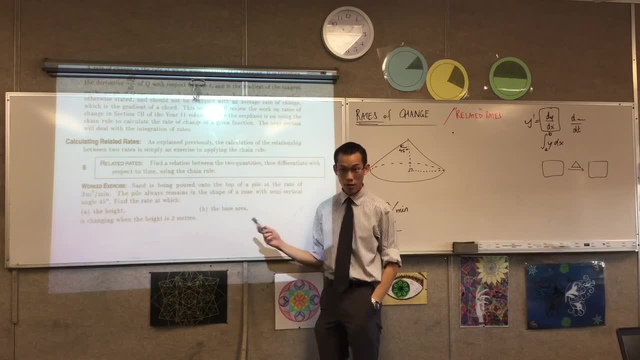 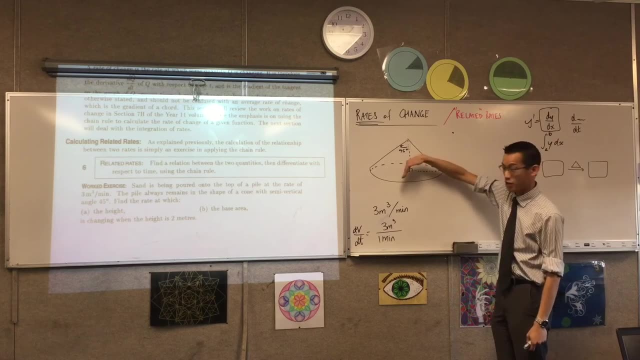 shape of this. There's two reasons. you can know They're describing the shape of the cone, not the shape of the not-cone. So the other angle- I suppose you'd say the angle of depression- is outside the cone. So you're not actually describing the cone anymore. 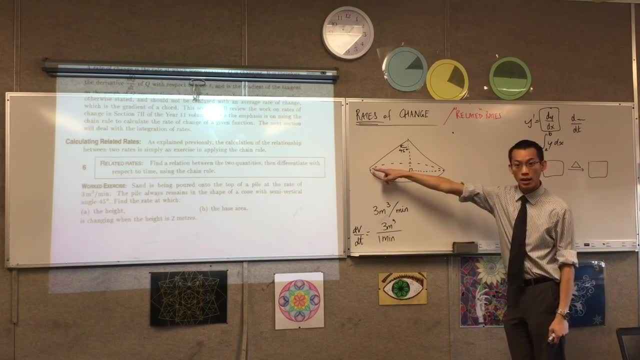 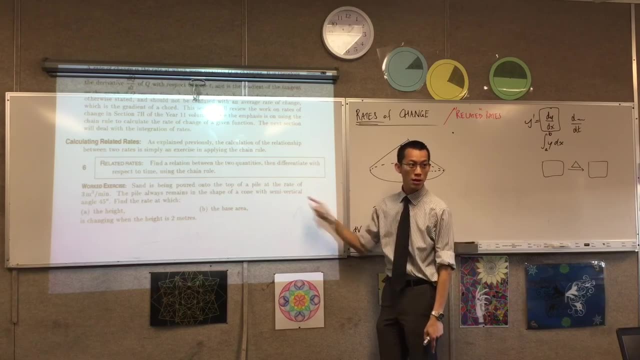 No, I mean the base angle. Sorry, say that again. The base angle of the cone. You mean down here? Yeah Well, that would come from this angle right Now. the reason I know this angle's up here and not down there is because it's a semi-vertical angle, so I'm measuring from the vertical.